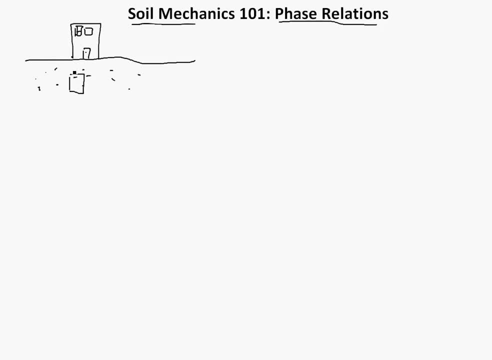 let's say we take a soil sample out. If we take this chunk out, then we get- let's draw a square. So we get, let's say, a square, And so basically we get a bunch of it's like soil and let's say: there's, let's say, the water table's here or something, The water table's under here, And so this entire thing's saturated. So you have here, you have. 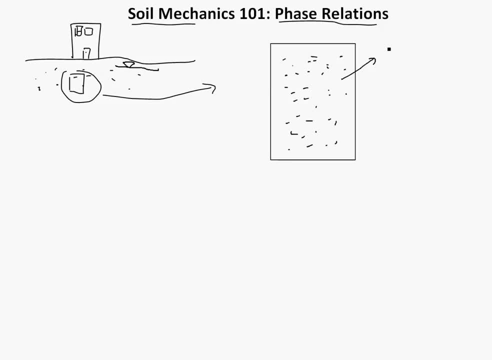 So you basically you'll have, you'll have voids or basically that are inside here, that are water or air, And then you have the rest is just solids, like rocks, gravel, clay and other stuff. So that's basically what this is comprised of, And then if we were to separate them, like we'll this is, we'll draw the phase relation. This is what a phase relation is. 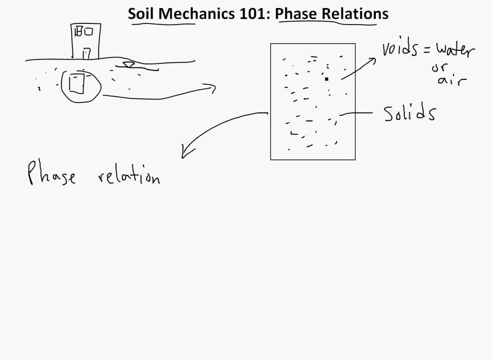 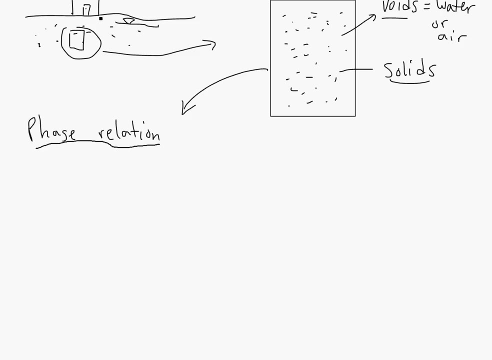 So yeah, because this is basically comprised of all, basically, solids and voids. Voids are just empty pores that you have stuff inside, And then we'll we draw the phase relation, draw this in terms of the amount of these. This is all what phase relations are. I'll just draw another one. So we draw another column. be the same thing, except now we're going to separate. Okay, we're going to separate the phase. Let's go here. 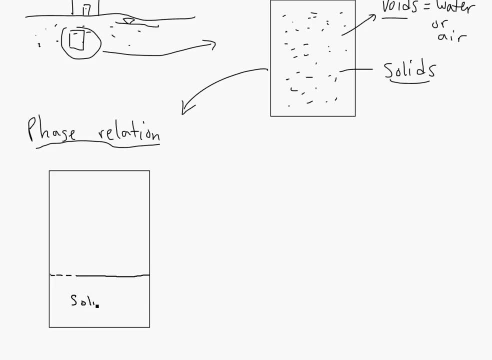 We're going to separate how much. Let's say this is solids, This would be solids. And then let's say here, Let's call this, this would be water And then this would be air. So we separate into three parts And let's just move this in the center, Move this, move this over here. Just I'll show you. We're just going to do some better drawings. 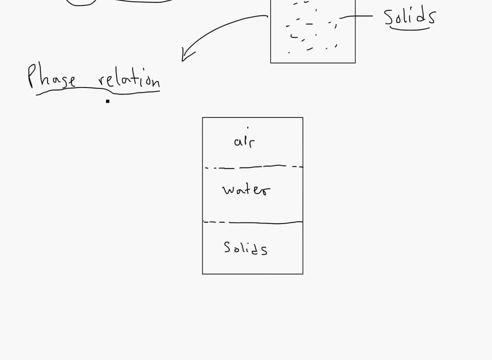 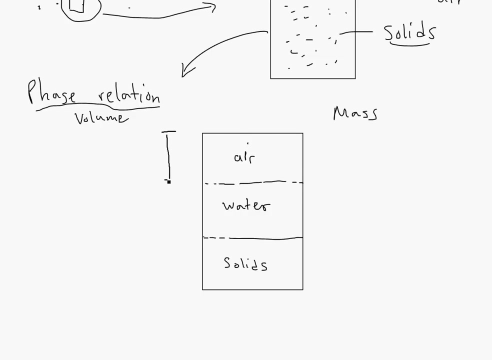 So let's say we have, if we we draw, we like we'll just measure out the, the weights. We'll go volumes here. Let's consider volume of this stuff here, And then we'll go consider mass. Let me just so, yeah, we'll consider mass here. Okay, so we'll consider that. So let's say we'll just draw it out here. Let's say for volume, We'll call this V air. 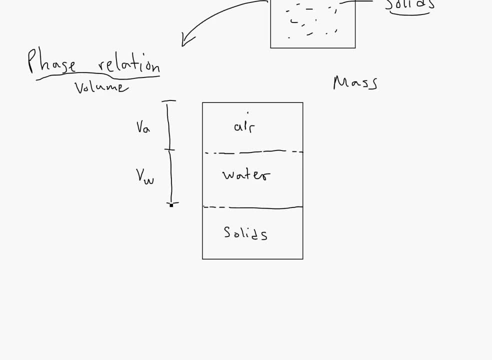 We'll call this V water, or VW, VA, V water, And then this will just be VS. So this is all we're doing is basically characterizing this soil in terms of its constituents- air, water, solids- And then we'll have, let's say this, this thing here will be V voids. That's V, that would be air and water combined to volume, And then here, this would just be V total. 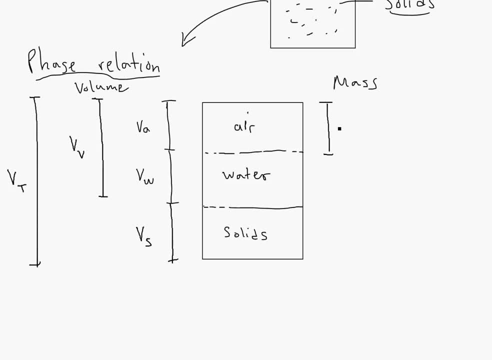 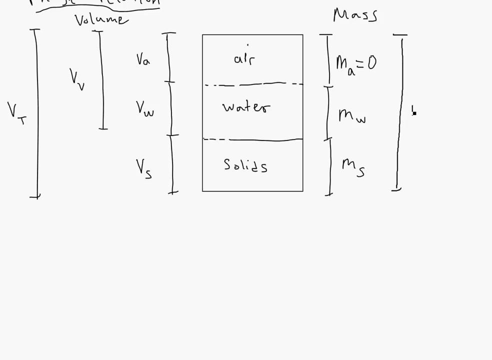 Right. here this would just be MA and this is basically zero. The mass of air is zero. And then we'll have here this is MW and then M solids. Okay, so we basically have, we define it in the total. here It's just MT, MT for total. 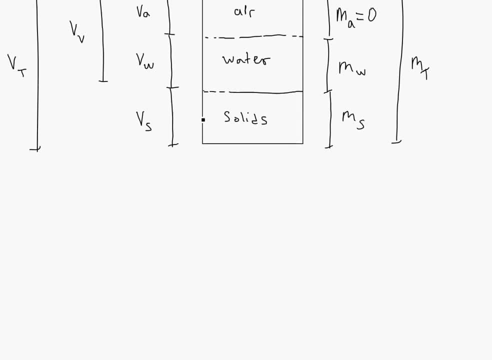 We. we just basically separate. That's all phase relations are. Now we're going to get some definitions based on these, Some important definitions that is used a lot in geotech or civil engineering Definitions. Okay, One of the most important definitions is void ratio. So void ratio- We'll define this one as E. That's void ratio, It's just all it is- is equal to the volume of the voids over the volume of solids. 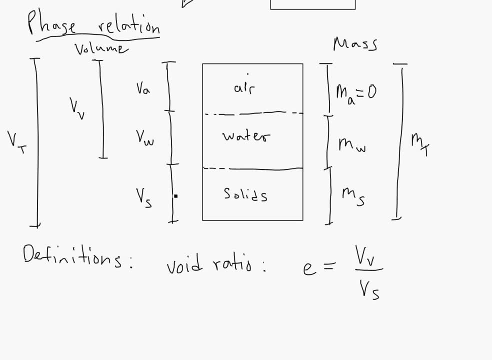 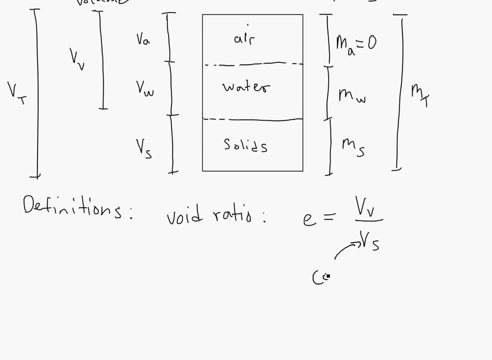 Okay, so that's all it is. so it's a ratio of this over this and it's, and it's good because you're dividing by a constant. this is actually constant. if you were- yeah, if you were- to compress it or what one of the solids won't compress and 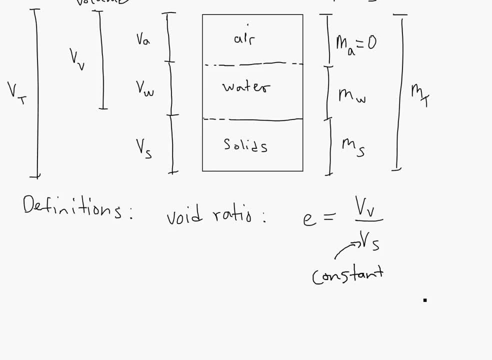 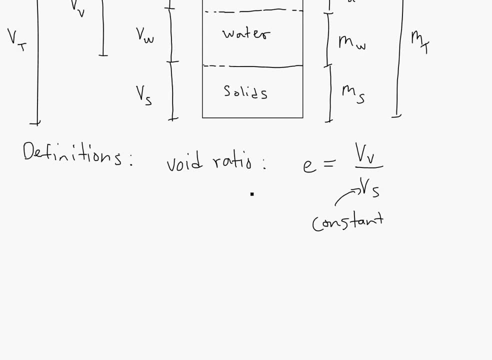 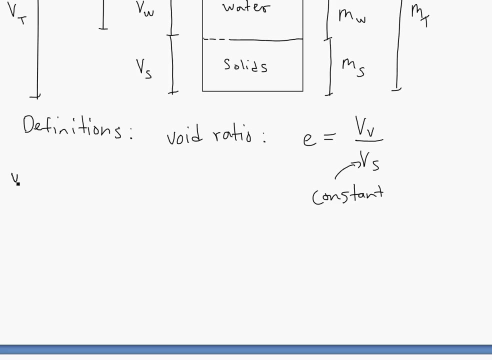 then basically water and air. so this is why it's very useful. so it's divided by constant and you'll see this many times in engineering and soil mining, geotech and civil engineering. it's all, it's all there. and another definition is water content. this one's called gravimetric because it uses- I'll show you this one. 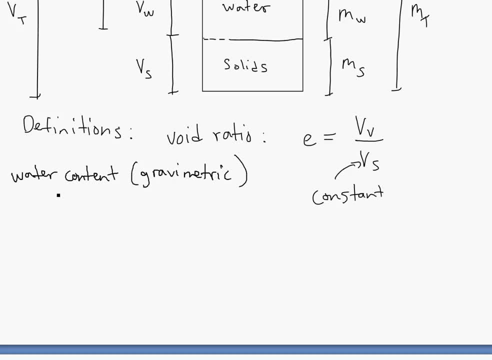 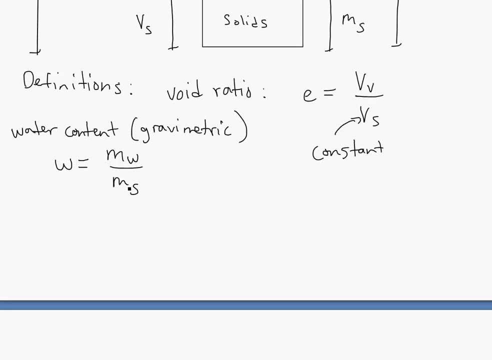 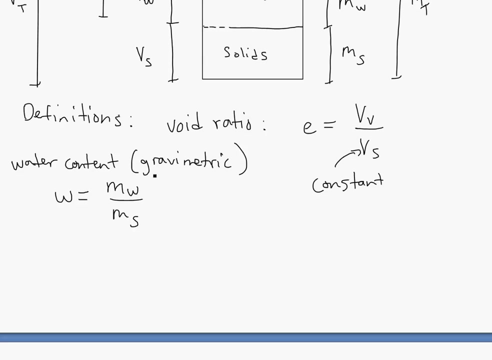 the gravimetric because it uses the mass, so we'll have water, no content. this is, W is equal to mass of the water divided by mass of water of the solids. so that's, that's basically what the water content is. it's the ratio of the mass of the water over the mass of solids and that's the 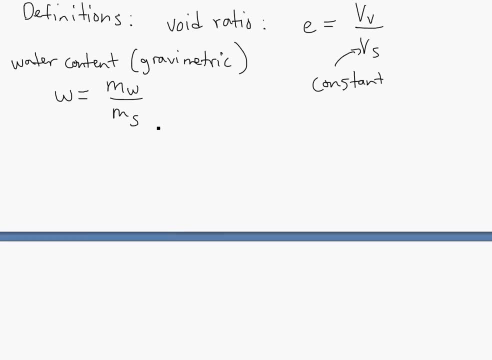 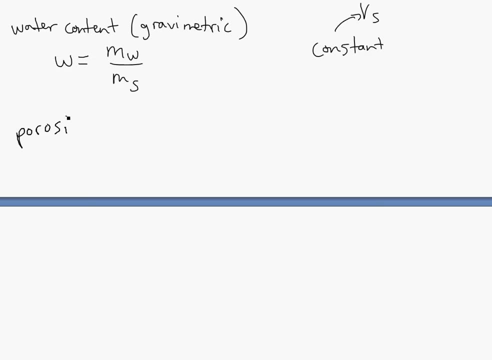 gravimetric. as you're using this, there's a. you could also can define it using volumes, but this one is used more often. another important definition is a porosity- porosity and this one's just defined. this one is this Greek letter. it looks like an N- I know what it's called- and then it's just basically defined: a. 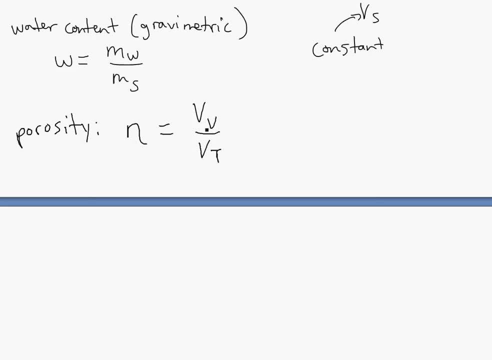 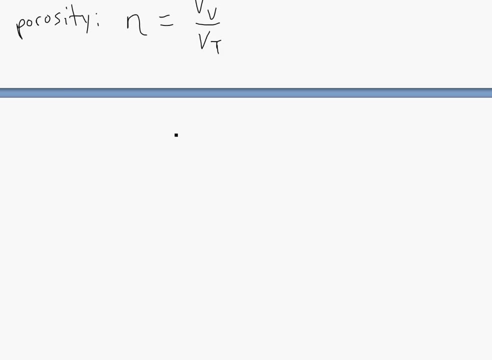 volume of the voids over the total volume. so it's just the. the salt is the ratio of, yes, the ratio of the voids to the total volume of the soil sample. ok, and and then another important one is degree of saturation. degree of saturation, and this one is, is just defined as s, z is equal to volume per. 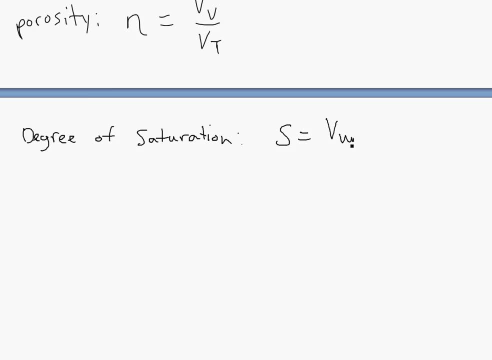 likelihood or the percentage of it being the to the volume over the total volume of. the verdict is always N: M the water. there's a race. it's the volume of the water over it's over the volume of the voids. so this is yet the degree of how much, so it's a hundred percent. 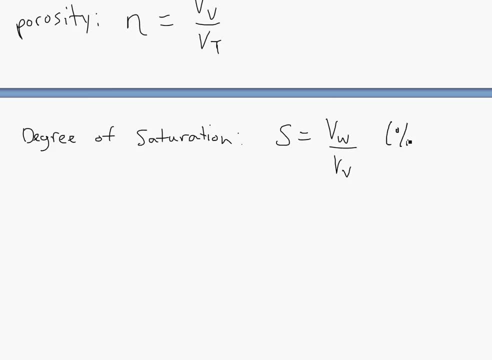 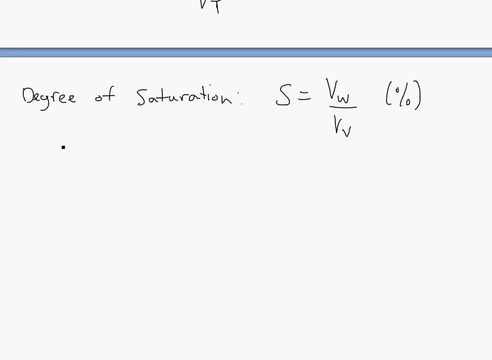 would just be: all the voids are filled with water and it's usually in percentages. so yeah, so it's basically the ratio of of how much water is inside the voids or the pores. okay, and then your, and then another. another important one is actually, say, dried dry density. we're gonna look into densities now. 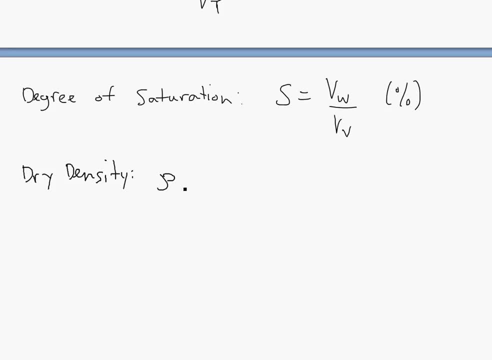 density. this one is a. there's a Greek letter row and then D subscript, so is equal to equal to the mass of the solids divided by the total volume. so this is the dry density. you can also have this one. here is the, the total density. this is dry. that is usually just consider the solids. 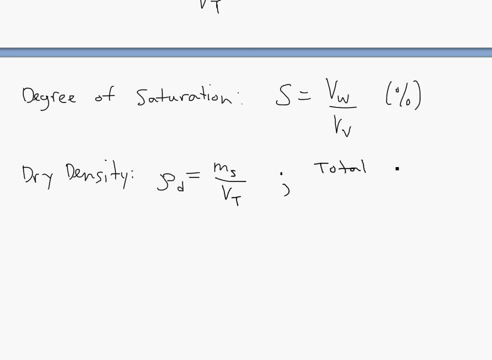 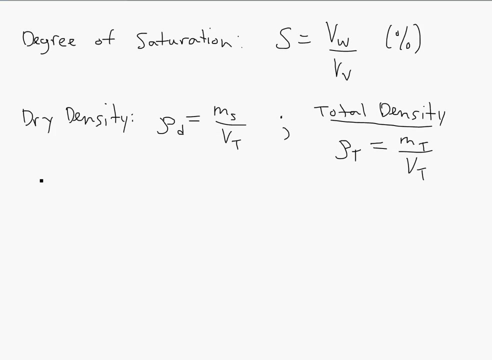 you can also have this one. here is the, the total density. this is dry, that is. or you could have say total density. so total density would just be: we'll call this row subscript T, and then this would equal to mass, the total mass over the total volume, and then and then, if we want just to density, the solids, no. 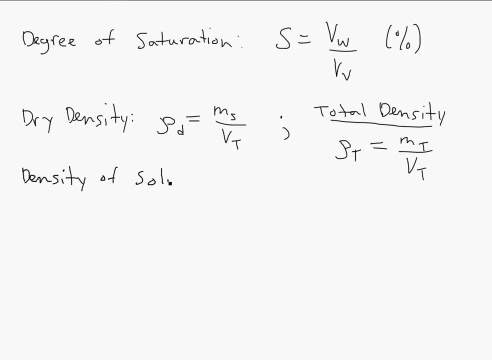 density of solids and density of solids, then we'll just go this row s equals subscript. yeah, row subscript s equals to, well, basically the. so it's basically equal to the mass of the solids over the volume of the solids. so then we'll just go to the volume of. 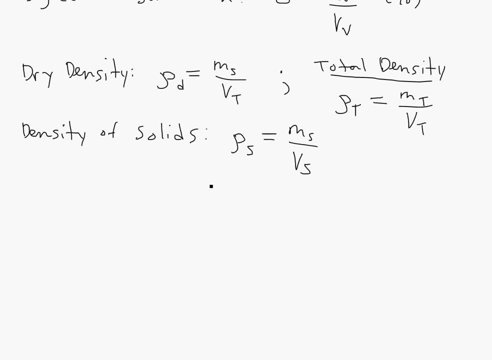 solids, so this is what it's usually using and density for, yeah, this one is basically a density fluid. this one is usually using a density fluid and it's of solids or just density. it's also used throughout, and relation between here and another one actually is a specific gravity. this one is very important as 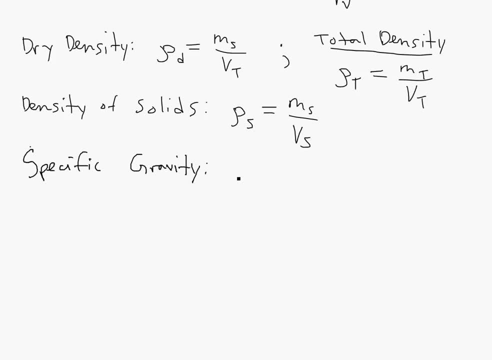 well, it's one of the more important ones. this and void ratio. this is, this is actually, this is equal to G, subscript s, and this would equal to. this is density of the solids over the density of water or h2o, and this is a very important 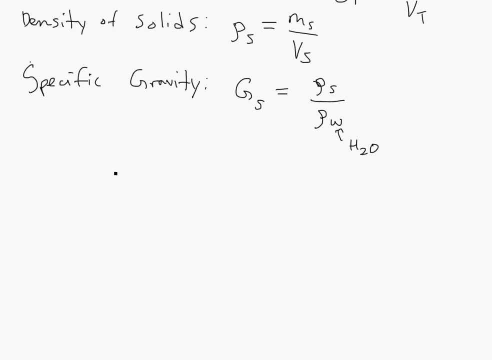 and used throughout. you know, and now we'll show you some and I'll show you some other, very like another. one other derived equations from these that are actually used a lot. let's say another one of this one is this: dry density could also equal to G of s density plus 1 over e times Rho W, so this one's an important 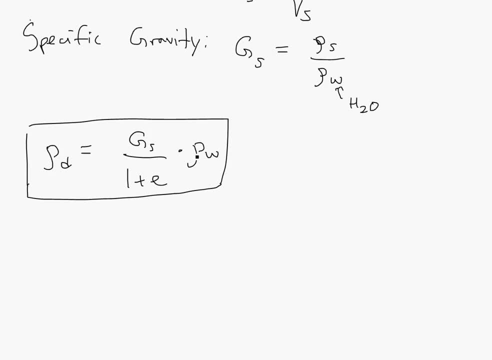 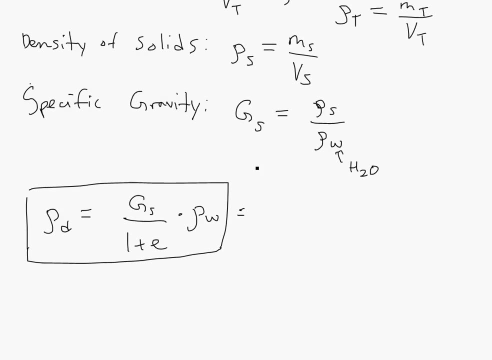 relation and you can, and you can even easily prove this one. all we do is, or we could prove that this, because this one is defined as this, we could easily prove it. to get there, we just go and we'll just go- that this is equal to Rho W. just put it there. times it by Rho W, this one's. 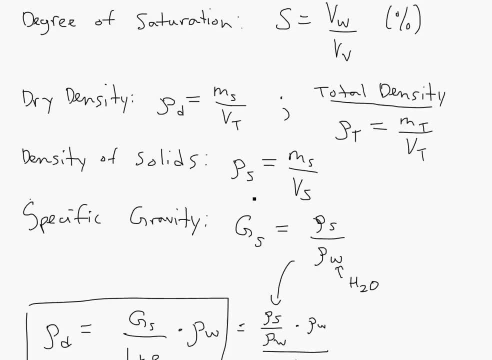 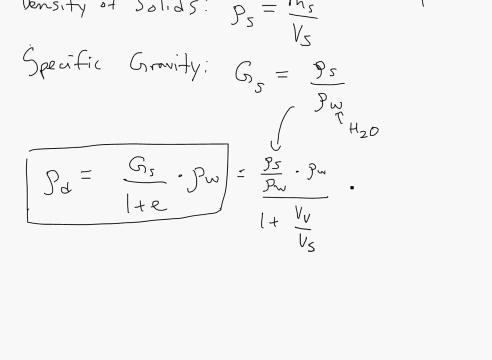 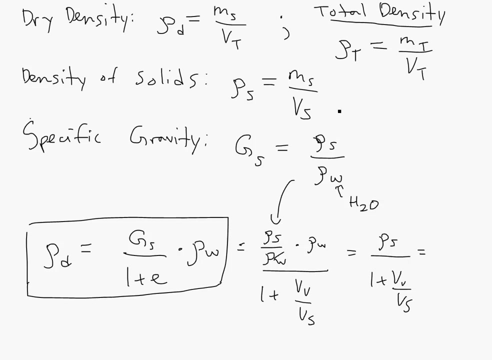 G of s, then this is 1 plus volume of what is this one? we have volume, voids of volume of s, V, V over V s, these cancel, these cancel and this will be left with this over 1 plus V, V over V s. and then this one, e is equal to this one is just ms over vs, vs, all over 1. 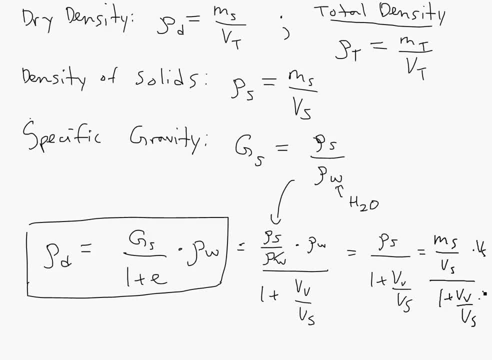 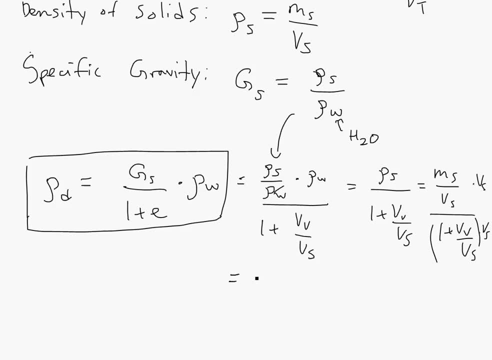 plus V, V, over vs. 3 times the top and bottom of vs and then vs. now we'll just get with this cancels and in this case we'll get equal to ms. well, this is subscript s, and then this is yep vs plus V, V and this: 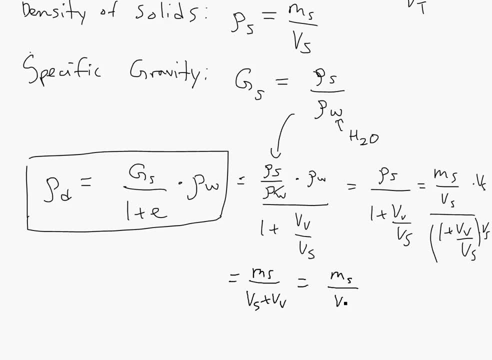 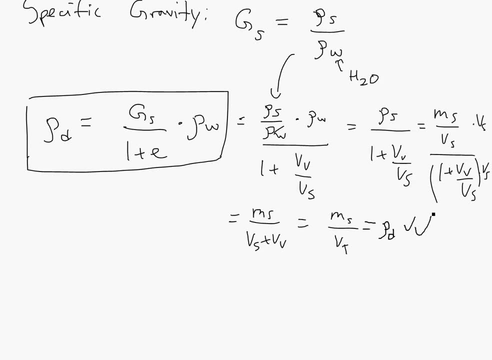 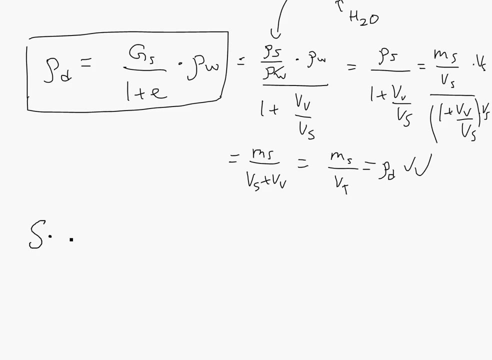 would just equal to ms over. this is the total volume for its both solids, V, T, and that equals to dry density right there. so equals definition. so it's right, and this one's a very important, and another important one is another relations s set degree of saturation times. the void ratio equals to water content times. 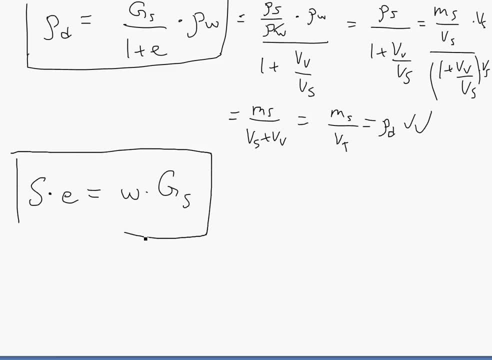 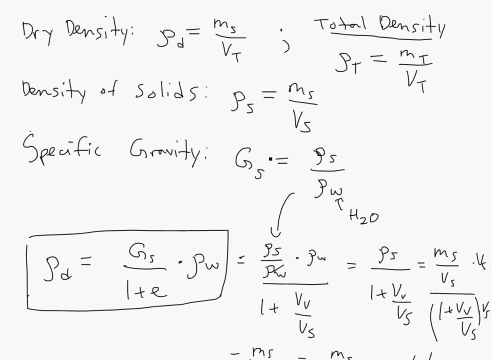 specific gravity, and this one you could easily yeah, this is a very important as well- you throughout geotech engineering and you can yeah, so these ones I just memorizing if you're in the field of this kind of engineering, but then yeah, in front of prove this. one degree of saturation is just, yeah, it's V, so V, W. 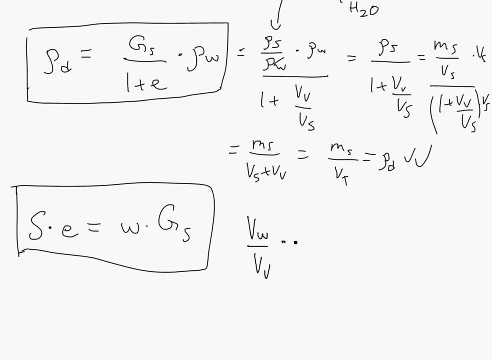 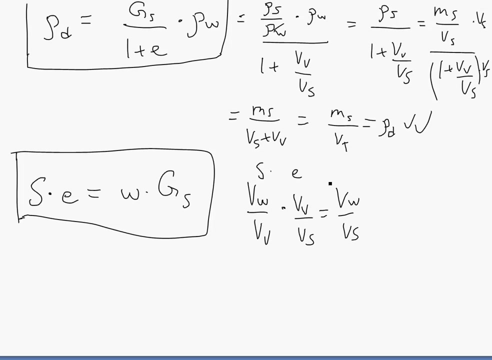 over V? V and then times void ratio, times void ratio, we will just get V? V over vs. this cancels. we're left with V W over vs. this is looking at the. this is s? e. and then we get V? W over vs. let me just make this better. so V W over vs. and then, if we look 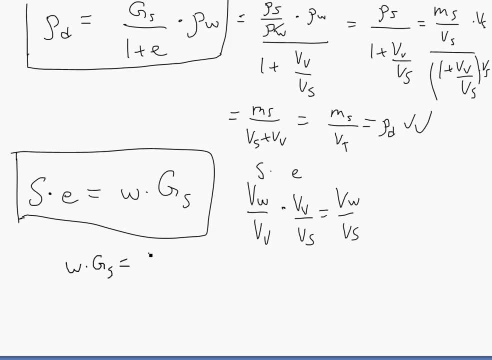 at W times, GS, this one would just equal to water content. this is just. this is so. water content is just an equal to mass of water over the mass of solids. then we're going to times by specific gravity, which is density divided by density, solids divided by density of water, and then